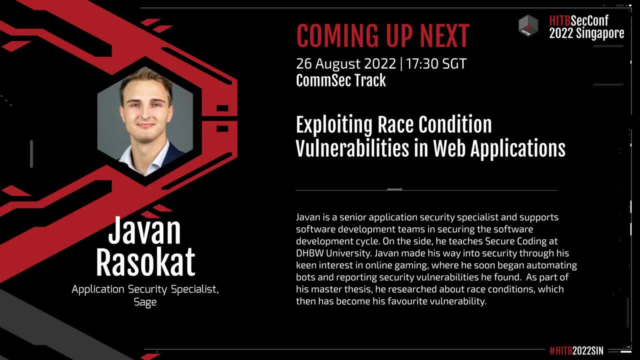 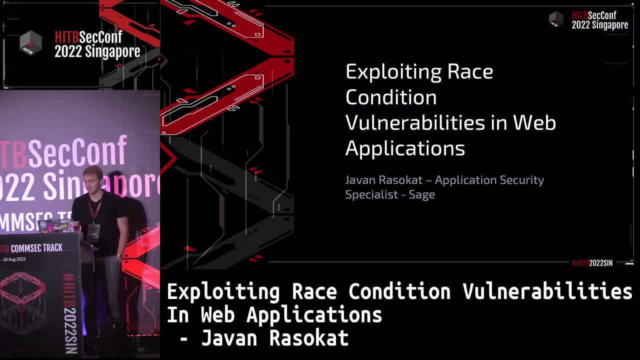 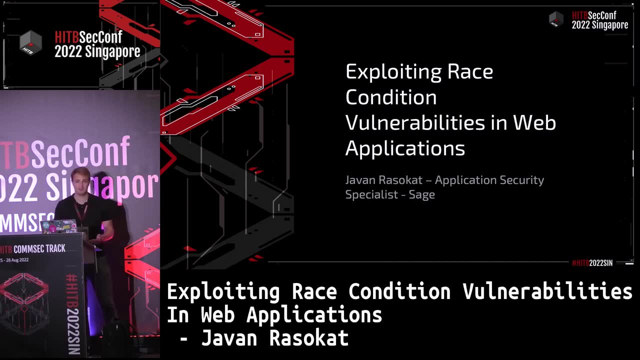 Yeah, thanks everyone for joining. My talk is about exploiting race conditions in web applications and I am very excited because it's the first time for me being in Singapore and I feel honored that my talk got accepted. Before we start with the talk: 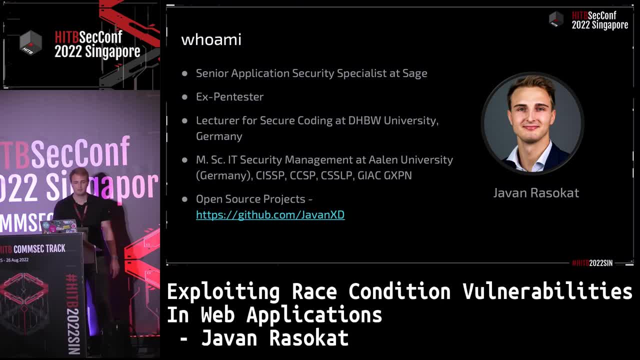 I want to say a few words about me. So I'm a senior application security specialist at Sage, So basically what I do is I support our software development teams in securing the software development lifecycle by integrating tools, securing pipelines, a general DevSecOps approach and shifting security left. 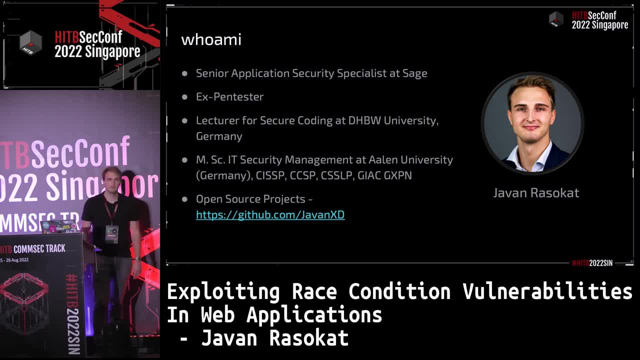 So I have a background in penetration testing and on the side, I'm lecturing secure coding on the DHBW University in Germany. I have a master's degree in IT security management, and what I'm going to present to you today, this talk, is a lot of. 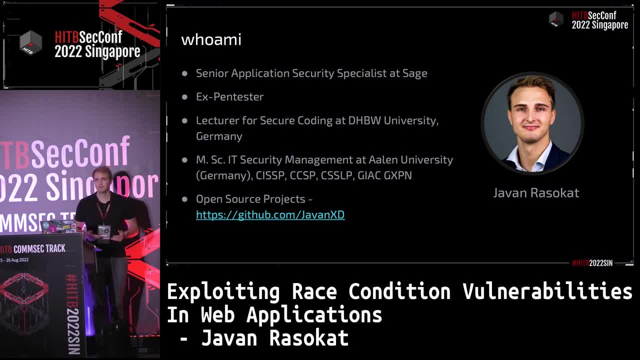 a lot of my research. I did as my master dissertation and I have a couple of certifications. I love open source projects. I have my own ones. I contribute to open source projects and especially in AppSec, for example, to Overset. 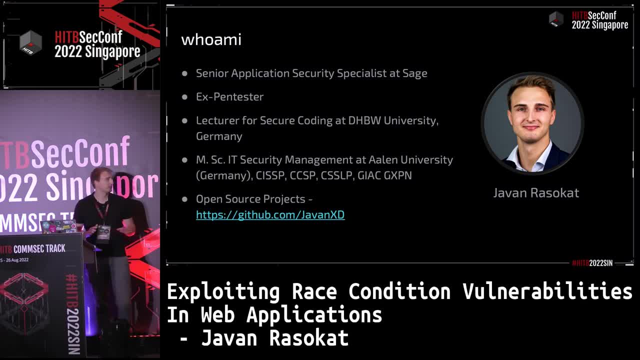 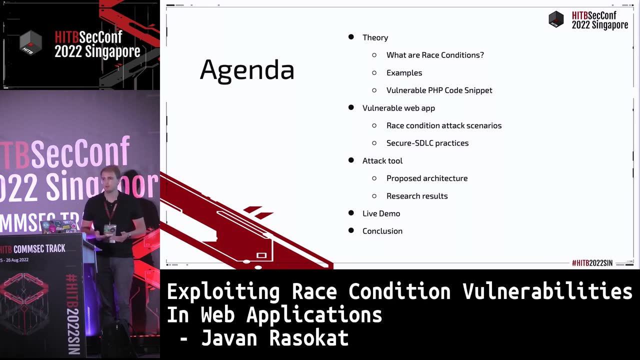 And everything you will find today in the slides and the tool I've developed is everything published on my GitHub repository. so all open source. Now the agenda today. so we start with a short theory about what are race conditions at all. Then we have a vulnerable web application. 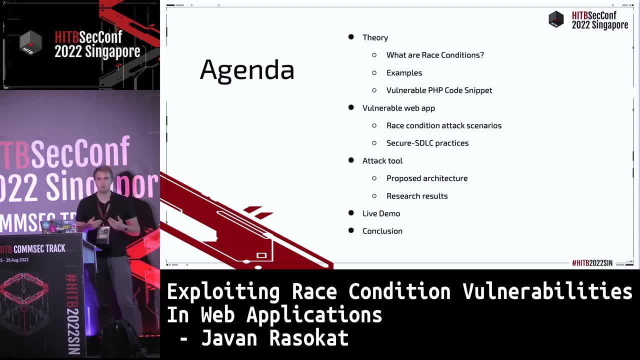 so this was implemented to show real vulnerabilities, real race condition vulnerabilities. They are all inspired by real bug bounty reports, by write-ups. So, yeah, we needed that vulnerable web application just to demonstrate also the attack tool which will be the next step. 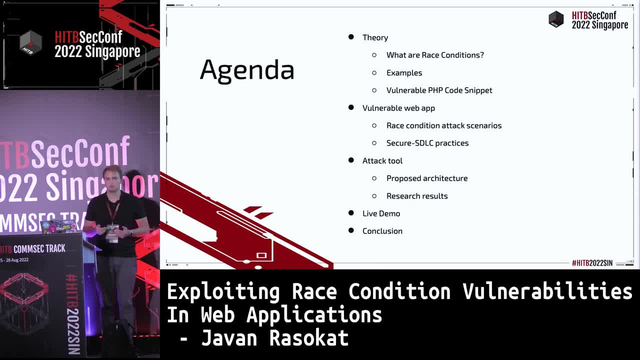 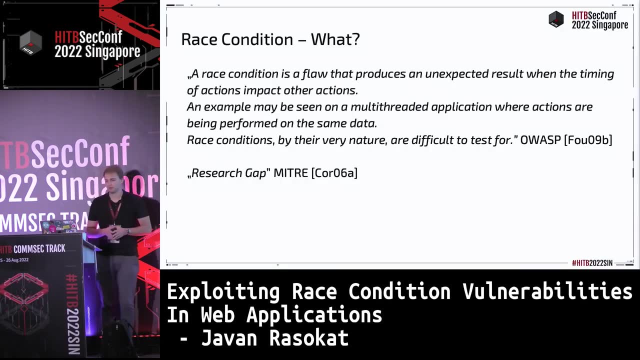 So I've developed a new attack tool to exploit race condition vulnerabilities and I'm gonna show you this tool in a live demo, and we wrap this up with a conclusion. So let's go to the theory. What are race conditions? So when you Google race condition, 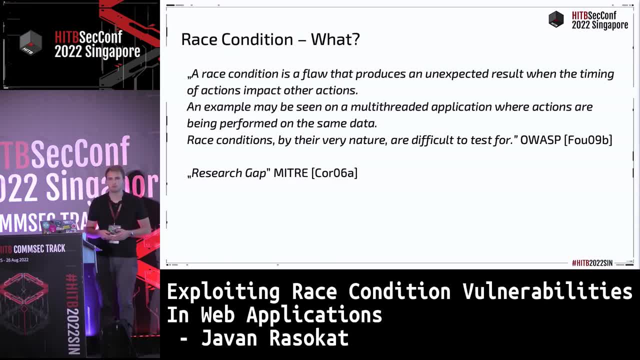 you will find this Overset definition. I want to focus on very last sentences of this definition. It says race conditions. by the nature they are very difficult to test for And I totally agree and that's also the impression I got up. 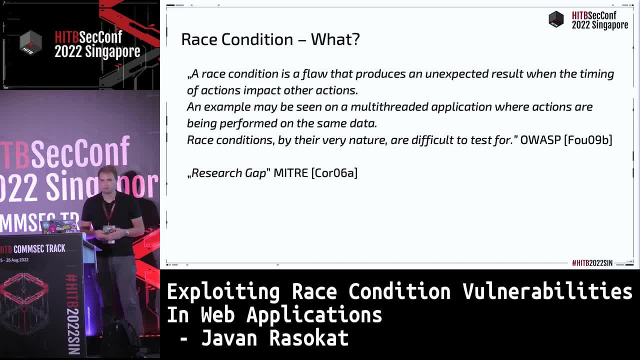 with speaking. some of you folks before this talk. So yeah, when testing for race conditions, it's all about timing, So it's very difficult to reproduce and stuff like that. And also MITRE they mentioned on their website also it's a research gap. 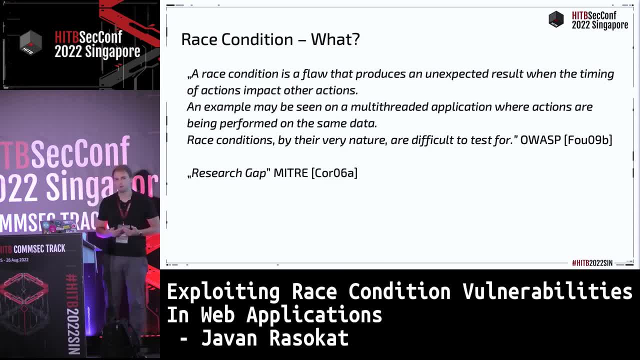 So I think there's little known about race conditions and there's still much to learn about them: how we improve our exploitation and our tool set to find them or protect us from race condition vulnerabilities And also, for example- I think it's often overlooked. 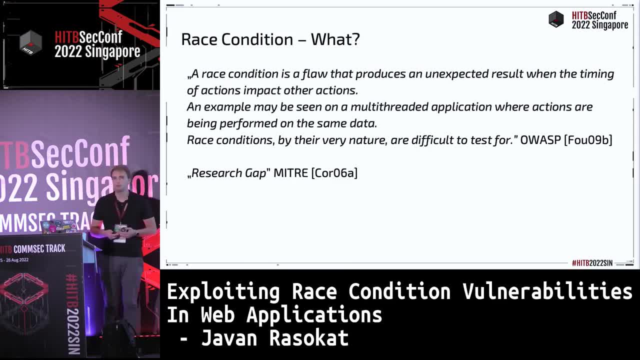 by penetration test because, for example, it's currently not mentioned in the OWASP testing guide. So yeah, it was mentioned in the OWASP testing guide in previous version, but it's not currently. But again, what are race conditions? I didn't explain it yet. 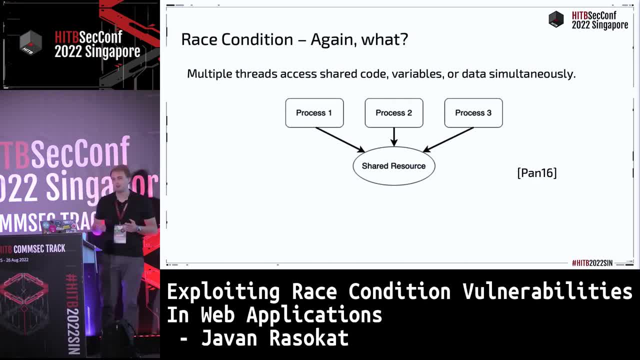 So race conditions? they are when you have a shared resource. This could be a file on an advice system, It can be data on database And you have multiple processes accessing or working with this shared data in the database And a race condition occurs when you have overlapping. 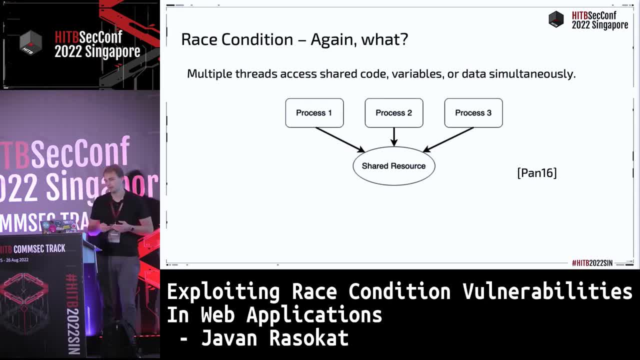 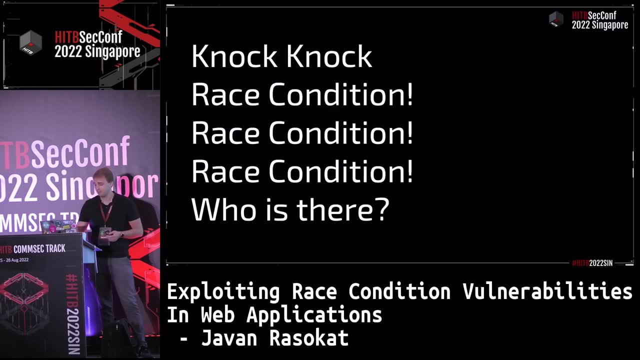 processes like multiple processing working with the shared data, and then you get unintended results. That's a race condition: Unintended results. Unintended results by multiple parallel processes working on the same shared data. So knock, knock. who is there? 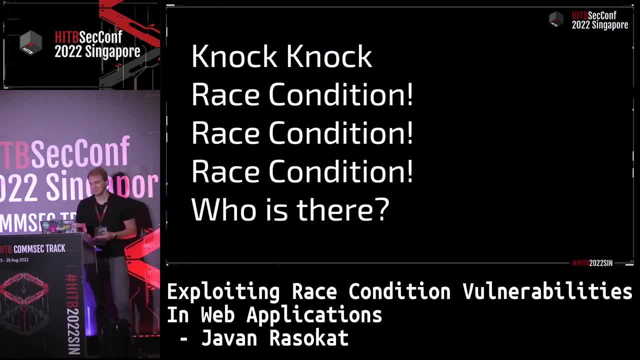 Race condition. So that's a common joke about race conditions. So this is one example how one could look like Like you have one process doing the knock knock and the who is there, And then you have another process jumping in in between this and doing the race condition. 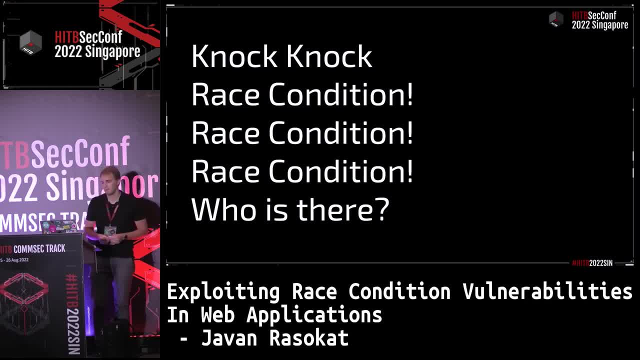 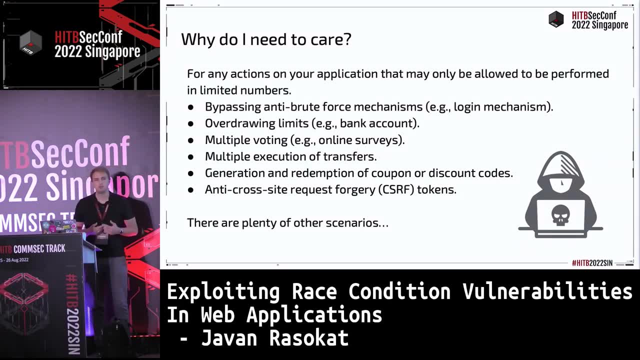 Like there is a time delay somewhere, But when does this became a security issue? Why do we need to care? So there are many examples and I will have a few of them for you. So it's often like, for example, when you would be anti-prude forcing mechanism. 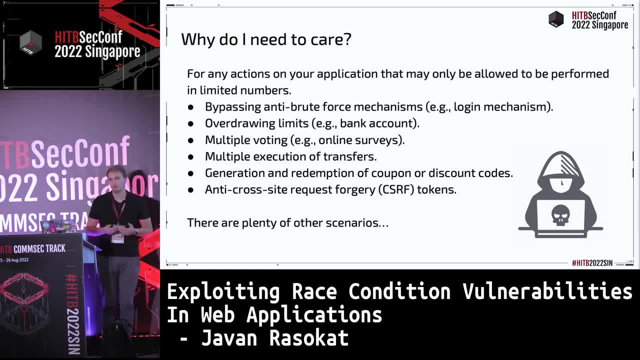 where you have, for example, a rate limit. So if you can bypass that rate limit, then it becomes a security issue. Or also other scenarios we've seen and also later implemented in the demo application. is, you can like, when you have a banking account. 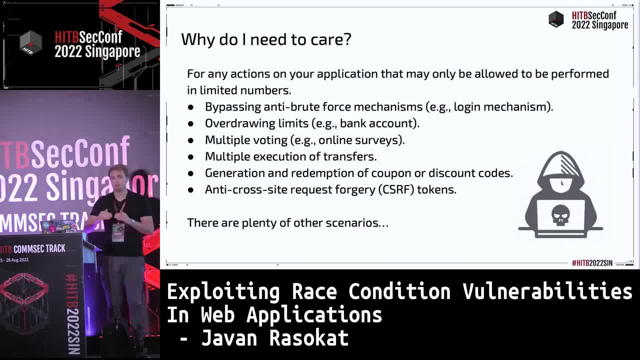 and you withdraw money and you can overspend your banking account. So there is this check which prevents you from overspending. by exploiting the race condition vulnerability, you are able to overspend your account And things like that, For example, multiple voting. 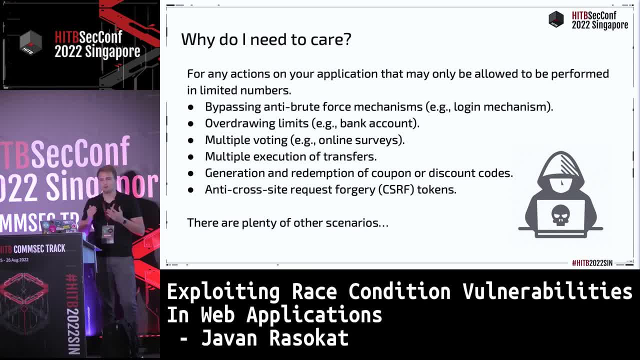 You know Twitter. you can press like on a tweet there and it's only allowed to vote one vote once per account. yeah, but actually this is a real vulnerability report. Twitter was vulnerable to this race condition. that's why I'm mentioning it. 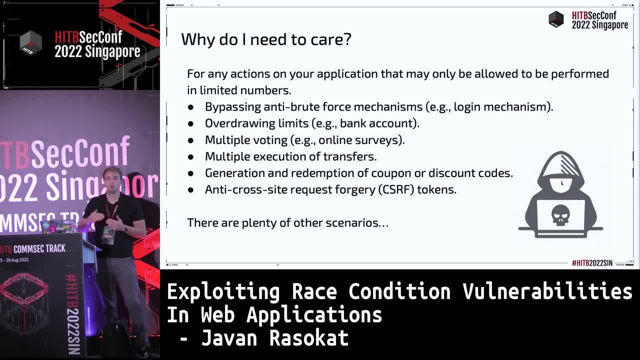 So if you are able to submit multiple votes so you can tamper this, that's also, then, a security issue And even cross-site reaches forgery. they are designed to be used only once. What if you can reuse them multiple times by exploiting a race condition? 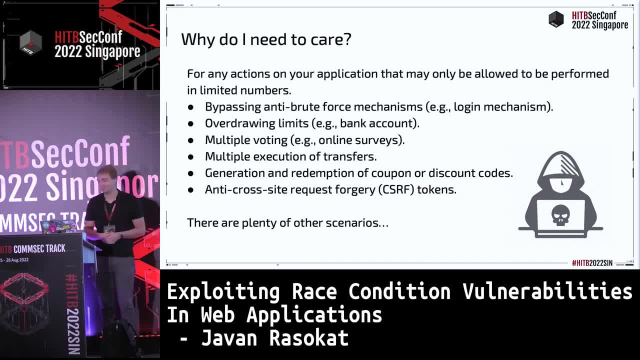 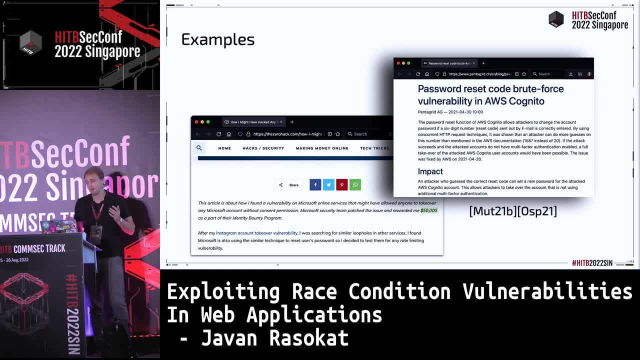 So there are plenty of examples. I brought two very big examples with me here in slides because they had a really big bug bounty payout. One was here from last year: AWS Cognitore. This was able to- a researcher was able to bypass. 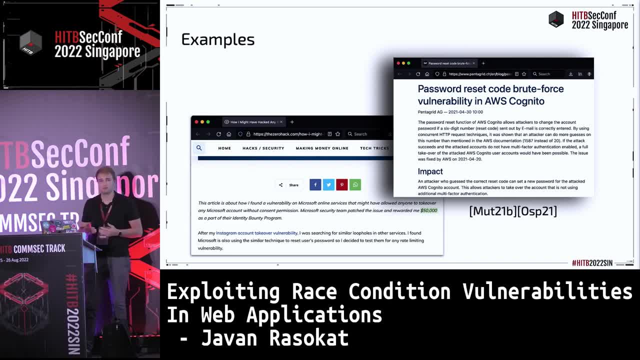 the password preset code, the rate limiting on this one. So they had a rate limiting for the bug bounty payout That you are only allowed to submit 20 times six-digit code and because of the race condition vulnerability, the researcher was able to submit. 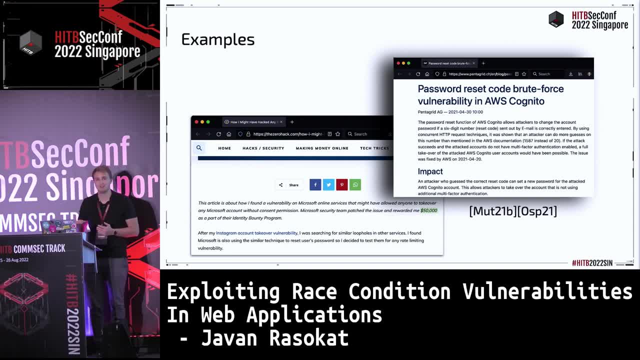 more than 1,000 tries of that six-digit code And also the other example in AWS and Microsoft in the password reset in the log in function. it was the same issue And this led to account takeover, which I think does have a very high or critical impact. 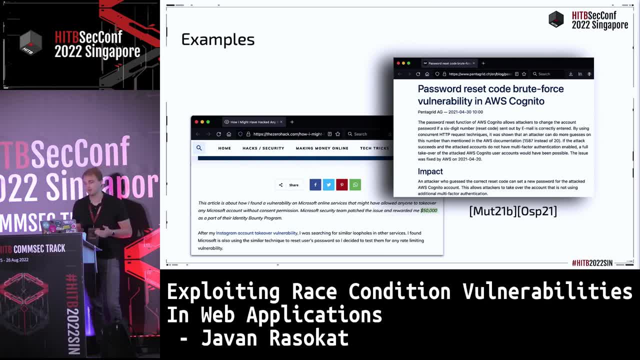 and that's why the bug bounty payout was that high. So for Instagram it was $30,000, and for Microsoft it was $50,000 for that researcher, And I just wanted to show you this example that race conditions can have a really high impact. 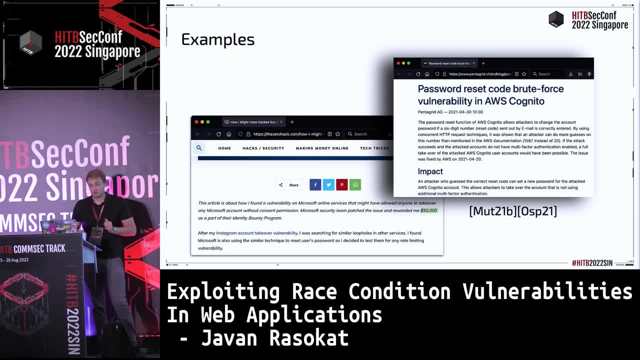 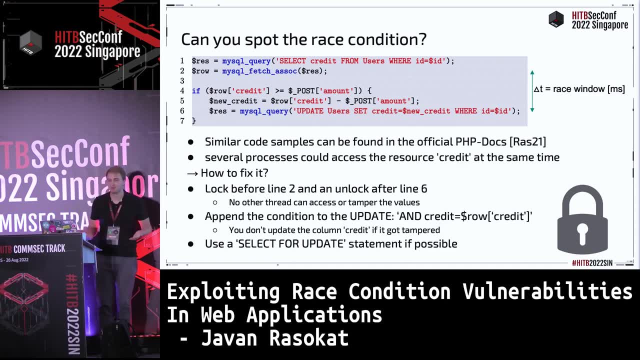 So I also brought a PHP example with me, a short code snippet, And my question is: can you spot the race condition? So for PHP it's by nature, it's a multiprocessing language And, yeah, when you see that code here I brought to you. 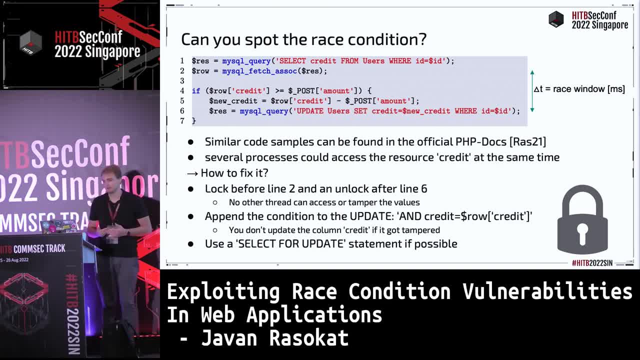 it's only the seven line of codes, but there's a race condition in it And very similar examples. if you go to the official PHP docs and search for functions for the MySQL functions over there, you will find these examples. That's what you see in StackOverflow. 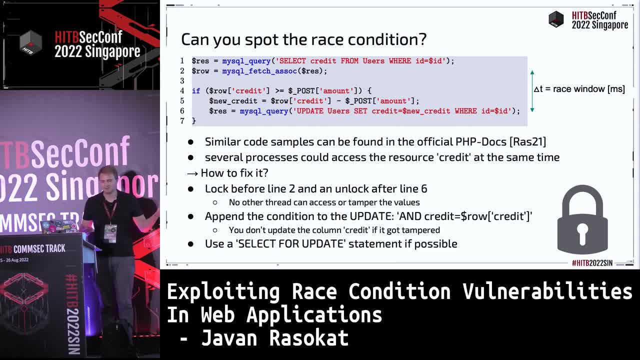 that's a real code snippet, but they are vulnerable to race conditions. And what developers do? they look something up on StackOverflow. they copy the code. So what does this code does here is it's like a withdrawal function. Like I mentioned, you have the table users. 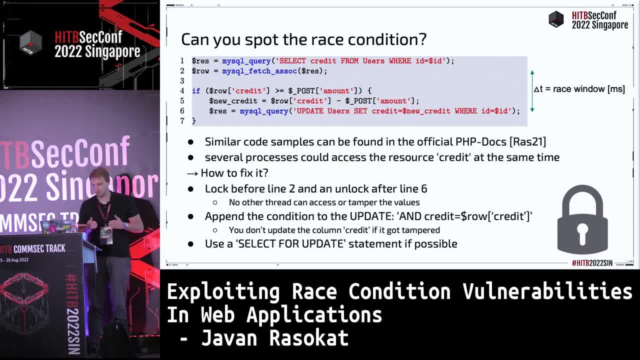 you have the credit and then on line four, you check if there's still enough amount to withdraw on your credit and then you withdraw the amount of money from your credit. and then you, in line six, you update the user's tables again with the new credit. 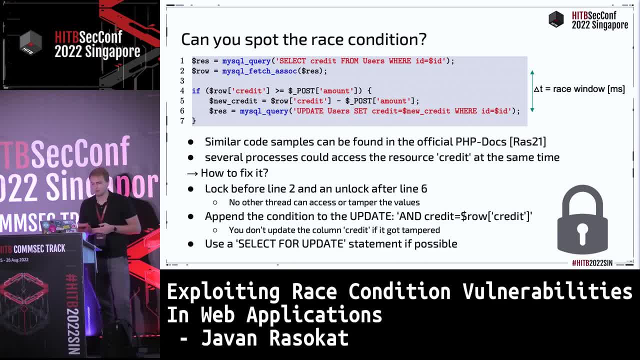 So a withdrawal function like a banking account, And, yeah, there's a race window between line two and six. So there are it's a very small time window which, yeah, another process could hit in, and then, yeah, there's a small delay, only in milliseconds. 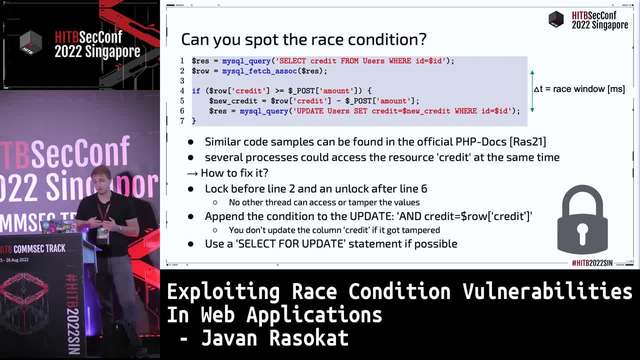 but if someone is sending multiple requests at this end point and he's catching the right moment, the right time, only milliseconds of time- then he could work on a not recent version of the credit table here, And I've only added three suggestions how you can fix this solution. 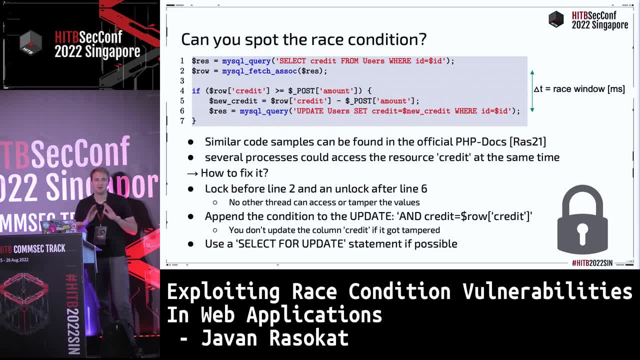 but I could have made a whole presentation only about preventing race conditions in different coding languages. So that's only a few ideas. So you could add a logging before line two and after line six, just that no one else can work on this shared resource at the same time. 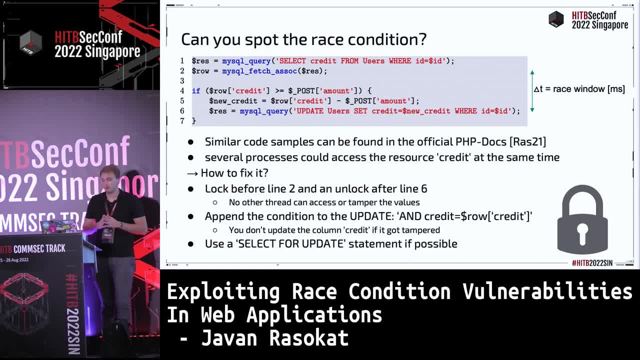 This is the most obvious one. I like solution two because this is like a fail safe solution. you can add an additional condition to the update statement. So where you compare, add an additional condition that you compare is the credit. did it tamper in the mean time? was it changed? 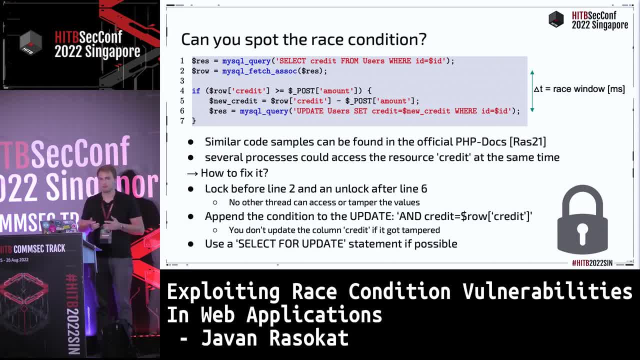 So then you could just say, okay, fail, It got changed to credit in the mean time, maybe by another process, And that's good. That's how you could also detect a race condition vulnerability. because you have this fail option, then you can say, okay, I had a sensor. 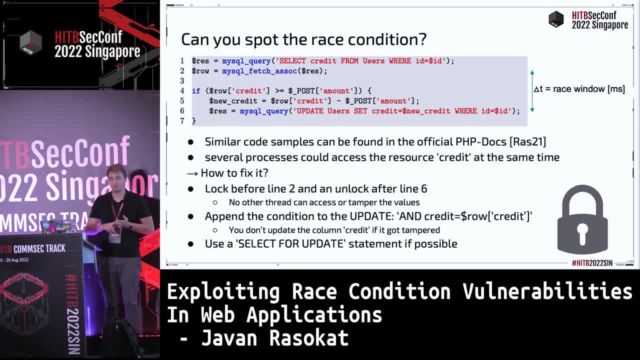 I had a detection point in my application and then I make alert and notify me that there was a race condition somewhere in my code. That would be a nice idea. And also, last option but not least, is you could change the whole code. 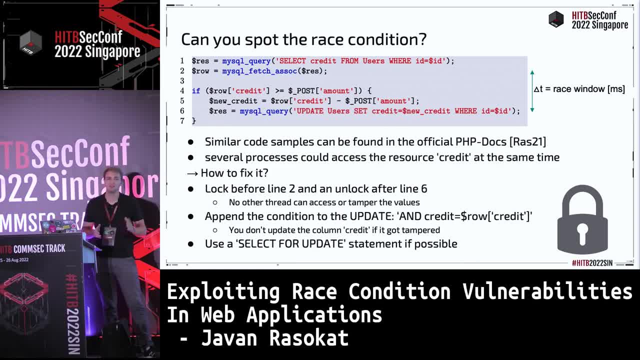 to select for update statement, if it's possible. I think in that case it would be possible to write everything into one SQL statement, all the everything, because if you have everything in one SQL statement, there won't be any time delay. 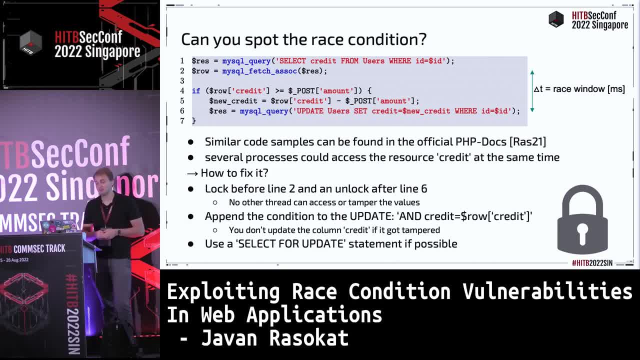 so you don't have a race window. Of course, if you have multiple SQL statements next to each other, then there's again a time window between them. yeah, But that's an example in PHP, and we could do this with other languages as well. 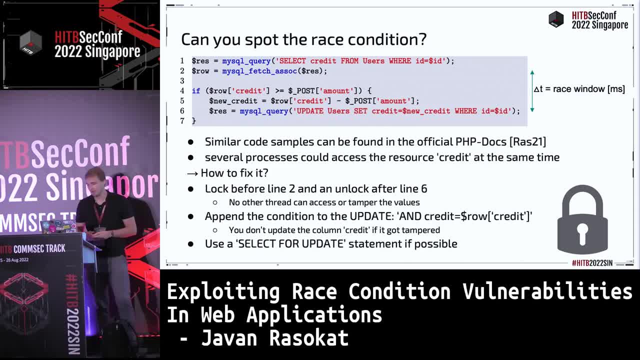 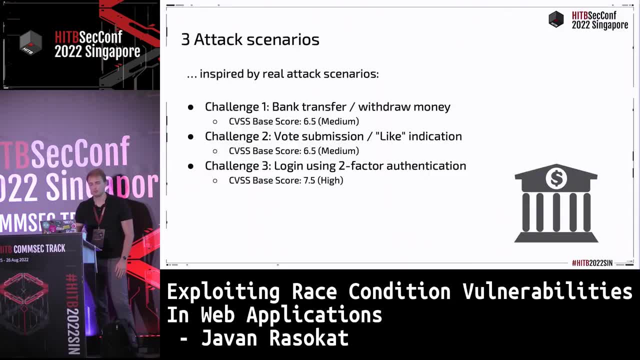 But yeah, So let's go to the vulnerable web application, the demo. So I've implemented three attacks and errors there, all inspired by real examples. The first one, challenge one, is to withdraw money. yeah, like the code I just showed. 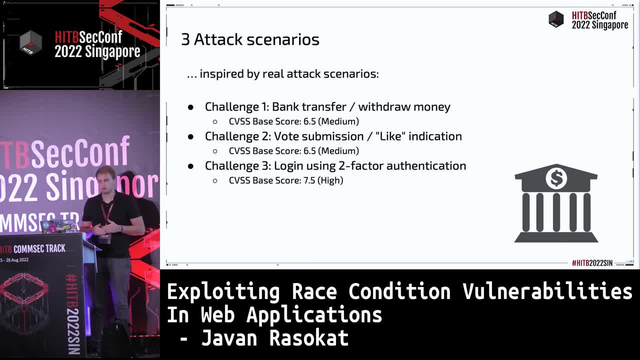 Then the challenge two: the vote submission. like the like indication- there's an example from the Twitter code. And challenge three is the examples I showed you from the multi-factor authentication that you try to bypass or rate limit it. So I also added a CVSS score on all these challenges. 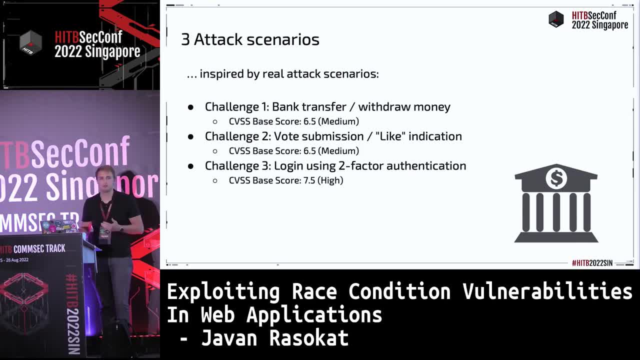 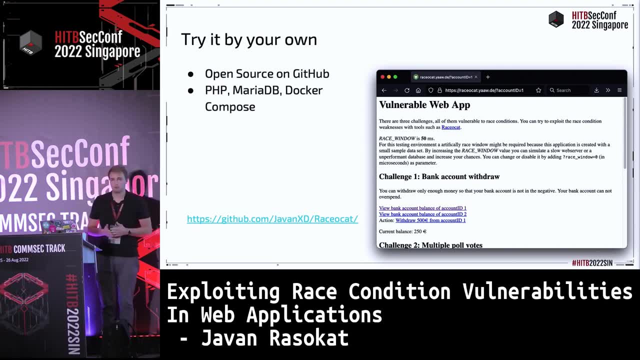 just to show you the different impact this could have. Yeah, So you can try it by your own also. So this vulnerable web application is published on GitHub. It's based on docker-compose, PHP, MariaDB, so the latest versions. 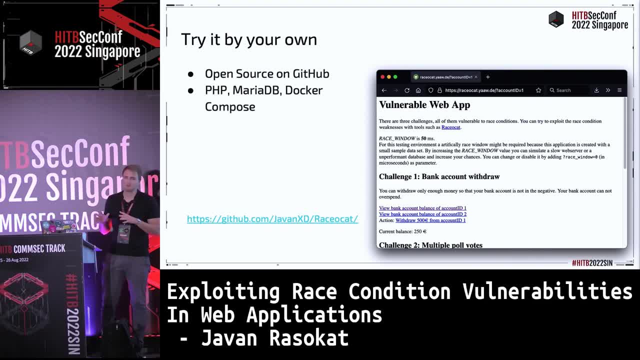 And you see, on the right side there's a screenshot from this demo application. I did not care much about HTML and design because the race condition is in the back end somewhere. It's in the PHP logic, So not that much design of the vulnerable web application. 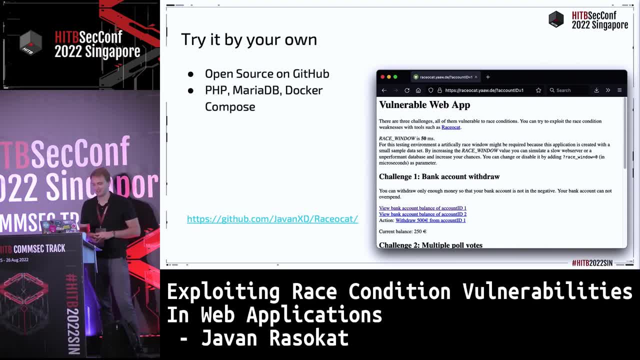 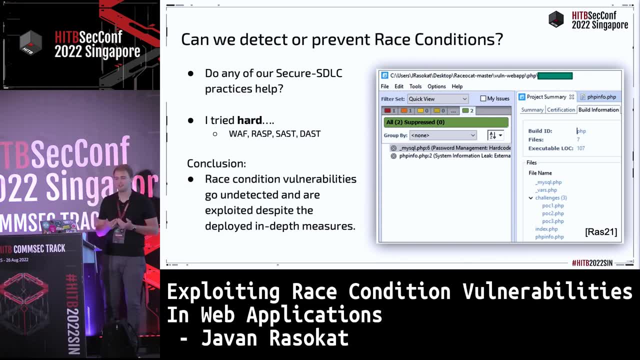 but it does its job, So yeah, Then the next one. yeah, I tried to detect or prevent that race condition I just implemented in the demo application. Yeah, you know, my job title is Application Security Specialist. I do these secure SDLC stuffs. 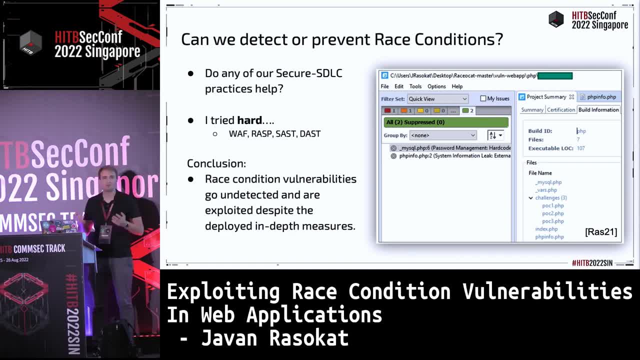 And then I tried very hard. I deployed everything I have Like. I have added a proxy, web application firewall in front of everything, Deployed a runtime application self-protection. I've run static code analysis. I did dynamic applications. 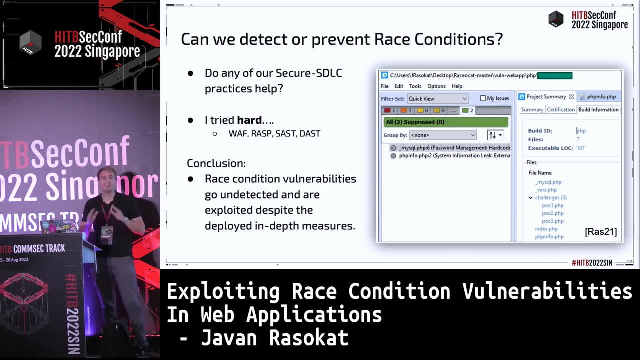 I did application security testing with overstep. I tried everything I could, But you see on the right side this screenshot from a commercial static code analysis. I don't want to drop any commercial names of the tools I've used, But yeah, you see, it detected some issues in my code. 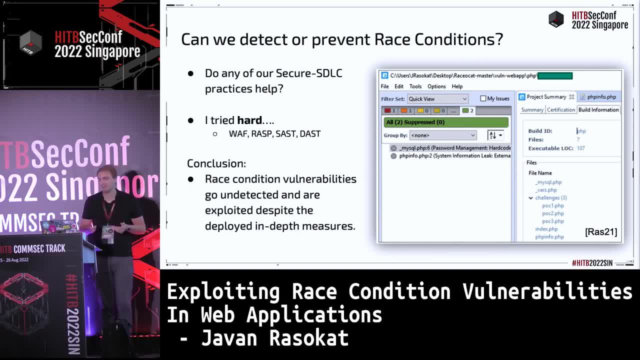 like a hard-coded secret. Of course it's a POC test, But it did not find a race condition vulnerabilities And I think they were pretty obvious And, yeah, And even the vendors. the static code analysis I used. 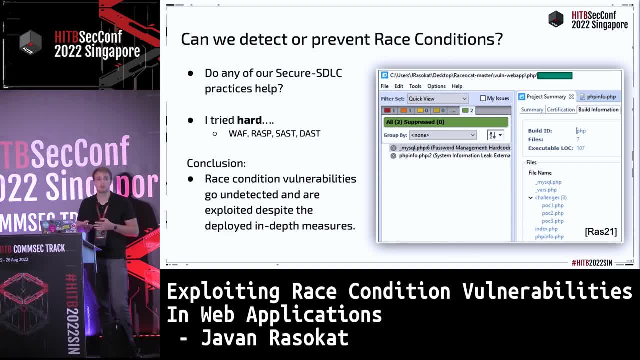 they claimed to detect race condition vulnerabilities in PHP, but they didn't. So, yeah, what can we do now? But I think this resource in the following conclusion that we still need penetration testing, We still need a human thinking about test cases. 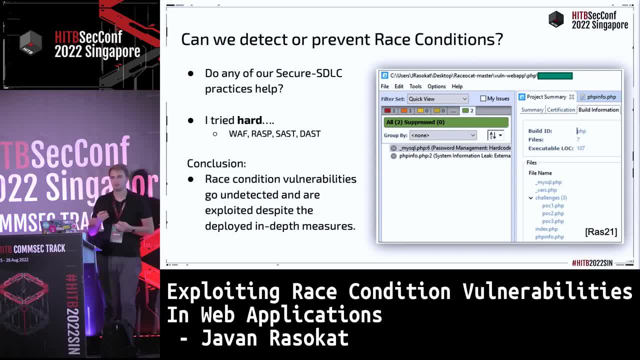 And thinking he knows the business logic, He knows best And you saw that there are a lot of ifs if you test for race conditions. Like you need a monetizing somewhere, like a withdrawing, It needs to make sense to exploit it. 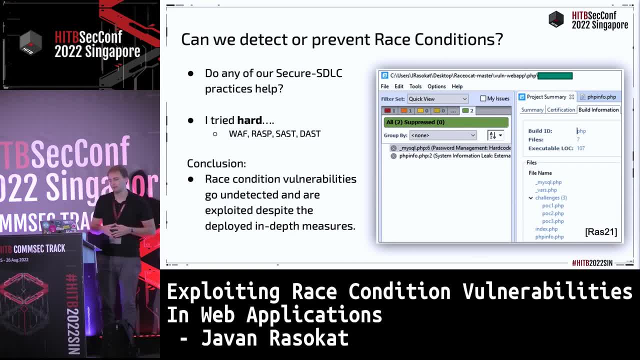 that it becomes a real security issue And I think it's only a human can do by doing tests. And yeah, a dynamic application security testing tool maybe sometimes can't, But I was shocked that the SAS tooling didn't find it. 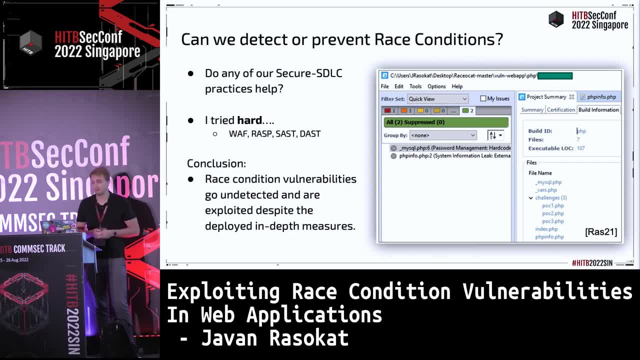 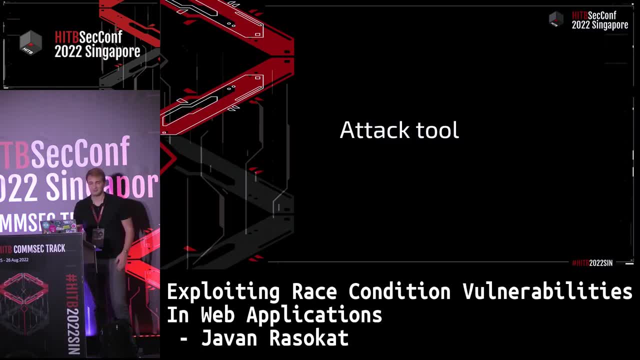 So I hope that at least that this would protect us. So let's go to the attack tool And try to attack what we just implemented- the vulnerable test cases- into our code, And before I do so, I want to also show. 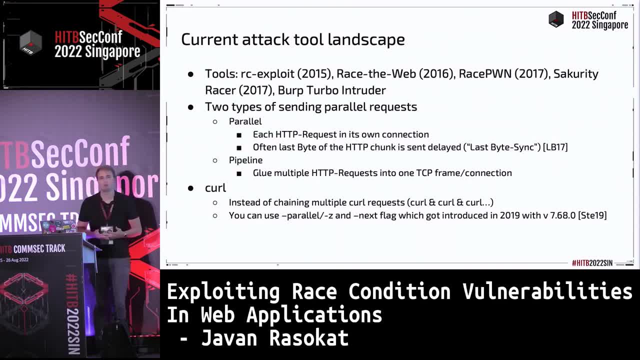 the existing testing tool landscape you have. Like there are common tools you can use RC Exploit. Raise the Web- It's Raise the Web He did. the guy who implemented it did a very good presentation on it. Raise Pawn Security Racer is a browser add-on. 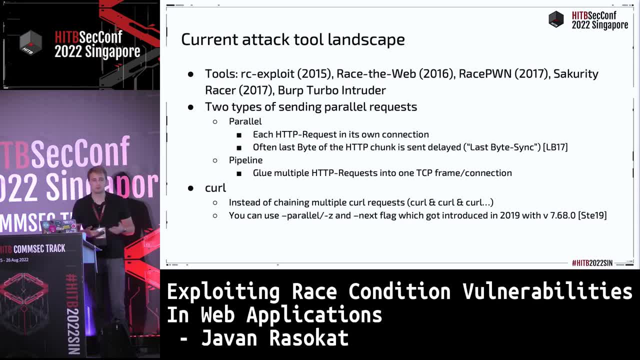 And, of course, Web Turbo Intruder- this is also very common- to test for race conditions. So all these tools, they have like two types how they work. The first one is you have a parallel function, which means each HTTP request you send. 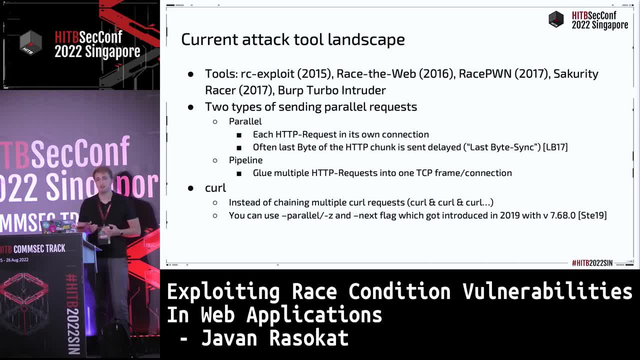 does have it's own connection. And then they use one trick- not all of them, but some do this one trick: that they have the last byte of the HTTP request and then you send this a little bit delayed and then this improves the. 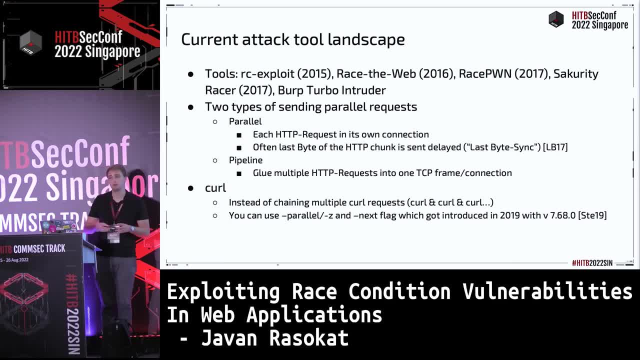 speed a lot, because you can preload a lot of requests and then send the last byte from all these requests at once, and then you have only a very small time window between each request, and that's why they work like this. and then you also have the pipeline function, where you can add multiple HTTP requests into. 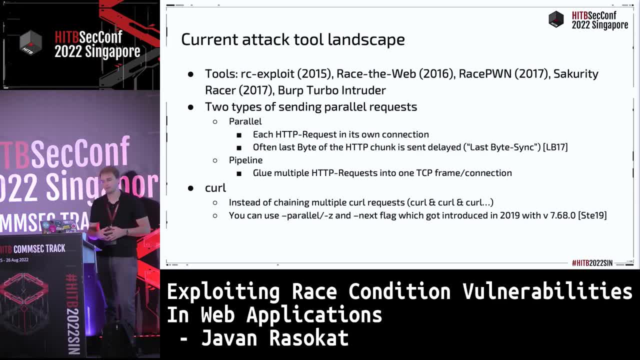 one TCP frame and it's also saves a lot of time. so, like I mentioned, risk exploiting race condition is all about time. you need a very smart small time window and that's why we care a lot of the performance of our sending our HTTP requests. and I want to mention curl because I I researched a lot. I back. 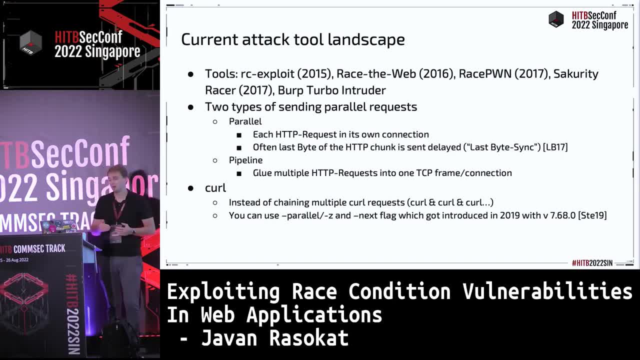 bounty reports. write us and everyone. some of these reports. they just change multiple curl. I mean this does its job, but there is a way, better option. you could use that, because curl introduced in 2019 a new flag. it's called parallel or minus set and that's this like sending multiple curl requests at once. it's very good and 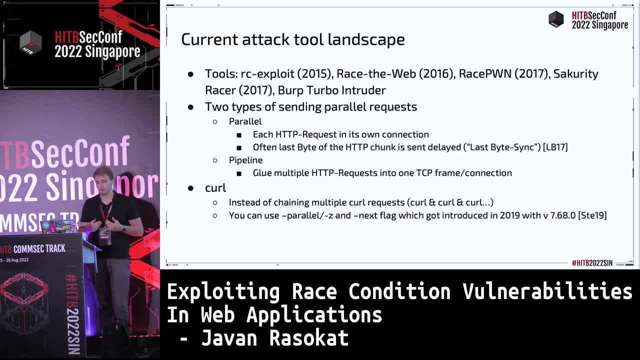 improves the performance of your request request if you use curl. so I haven't seen this anywhere. that's why I want to mention that, because it's still an option to to use curl with the parallel function. so but now, now I want to present you to attack tool. I've developed some. 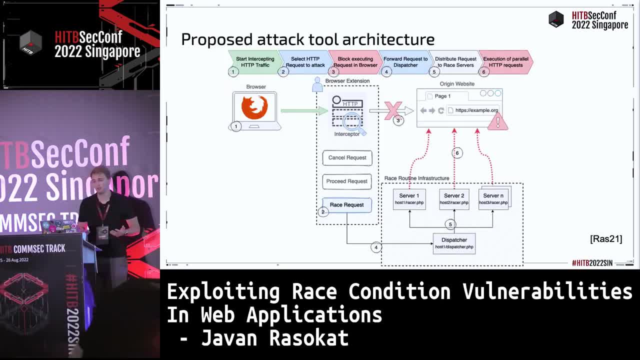 improvement from the existing tool landscape. so that's my proposed tool. basically, it's a browser extension to intercept the request while you work with the application and then you can select a request you want to attack, like could be any API call of your application you selected, forwarded to the 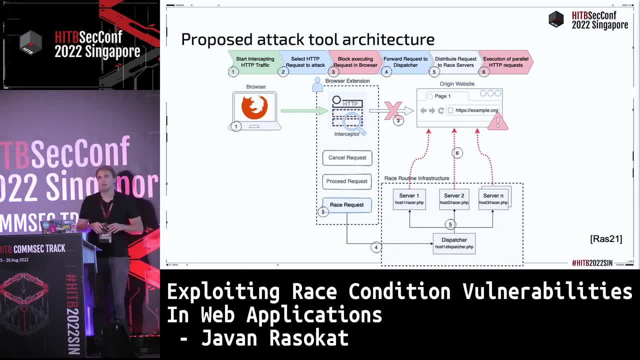 tool and but it's. it does also have over step integration, so you don't need to use the browser add-on you and it also does have a API so you could integrate it into CI CD testing if you want. yeah, so it's just about selecting the request. 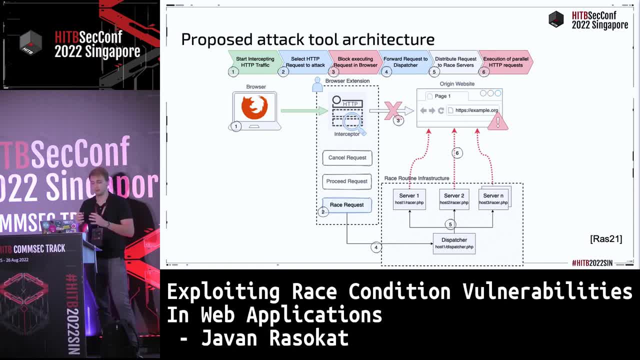 you want to attack and then you forward it to the, to a dispatcher. so now you need a race in a routine infrastructure to set it up. so I wanted to. I didn't want to run this on my local machine. I wanted to have the best performance. I. 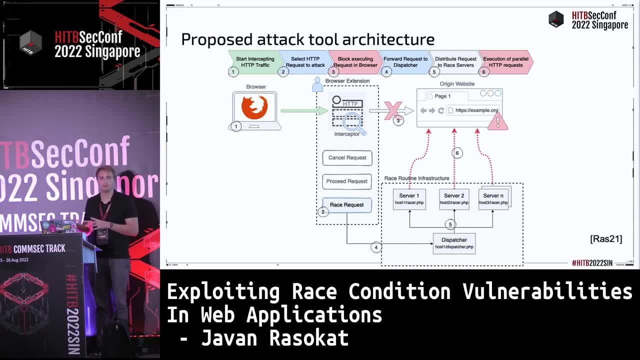 could get. so I wanted this to be on a data center anywhere deployed, maybe next to my target that I want to attack because I want a very short delay on everything, and and then was also different from the existing tool set. I want to take use of multiple servers doing this, multiple servers sending. 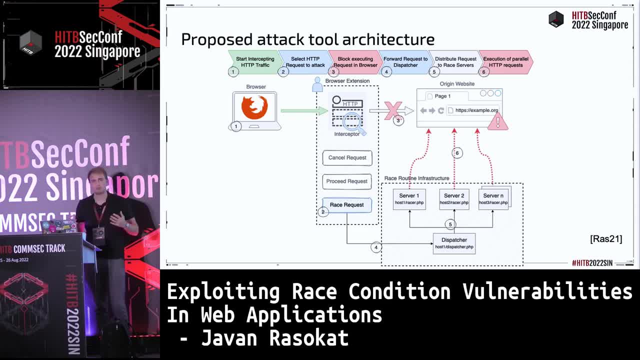 parallel requests and try to get this request that with a very short delay in between. so that's, um, yeah, what you can see here. like this, this routine infrastructure, this dispatcher is forwarding to the other service and then the request gets sent in parallel with a very short delay. 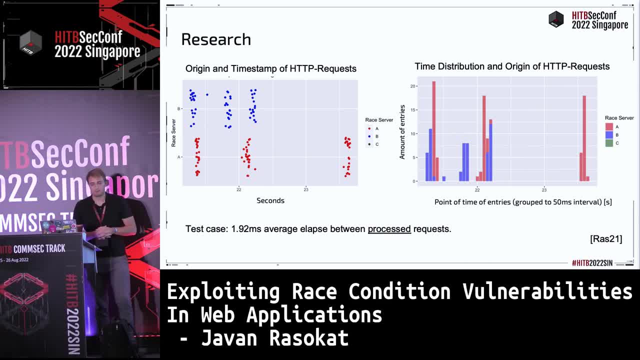 yeah, this, that's the some, some stats here from from testing this out. so what you see, in that case I use to race servers to send it to server sending parallel requests and you see there was an overlapping. so each point means one HTTP request processed on the target and I wanted to have a very 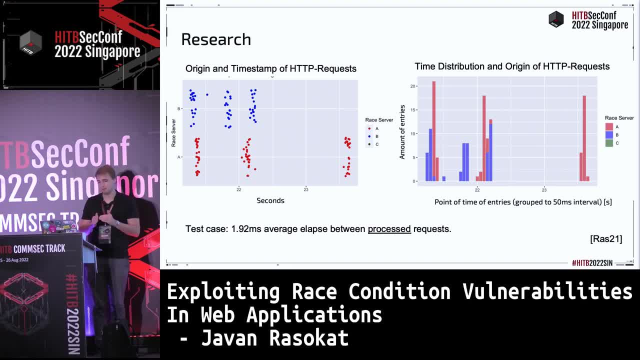 very short delay because it's all about millisecond, milliseconds here and you see, by using multiple servers you can get more requests, process on the very same time on your target and it makes explosion like successful exploitation makes more success the probability problem. so, yeah, you see, in an 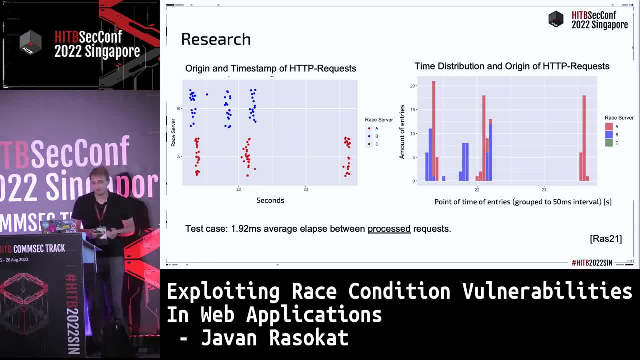 Thanks for the grabs. An average for that test case was a 1.92 milliseconds between each request that came to the target. I didn't use the metric request per seconds or something. I wanted to see the real time on the target between each request being processed. 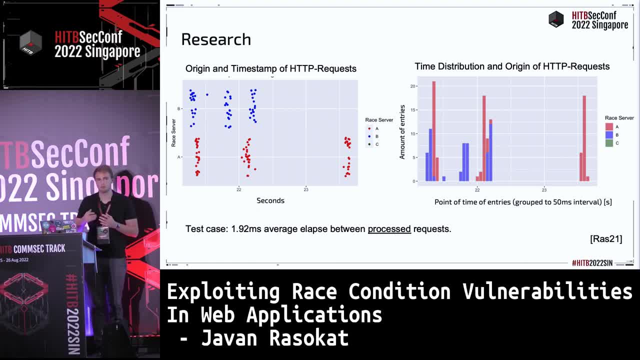 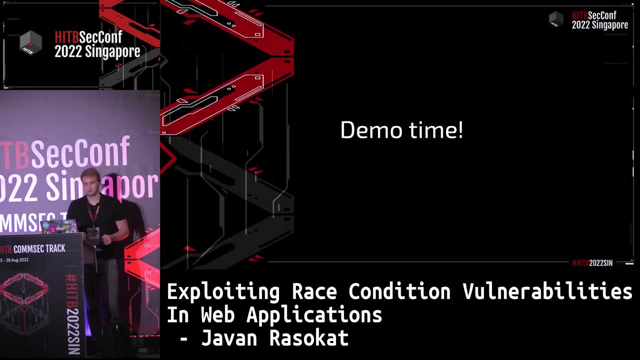 because that's what matters when you exploit the RAISE conditions- the time on the target- and not what the tool is able to send, how many requests to do. It's only the time of the target And yeah, good, Yeah, let's take a look into the demo. 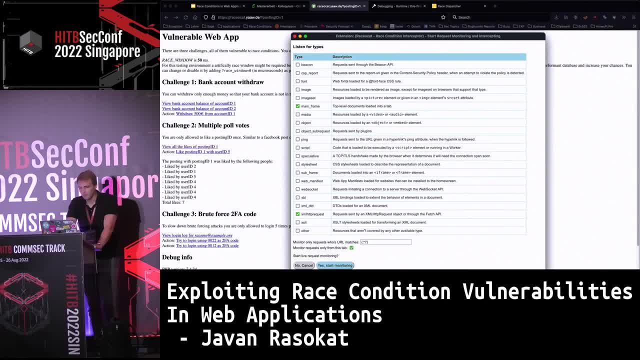 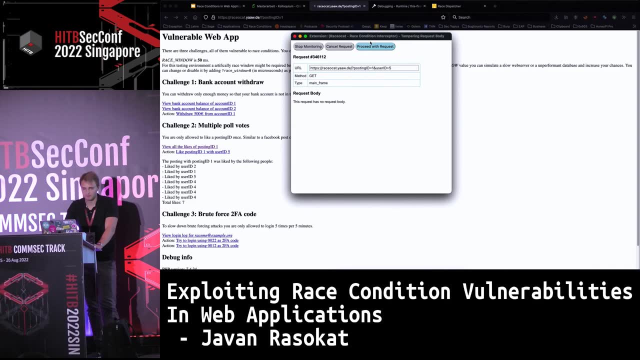 how it works in action. So we have this vulnerable web application. This time I show it to you with the browser add-in And I start the monitoring on the browser add-in. So you see, on the left there are the challenges I've implemented. 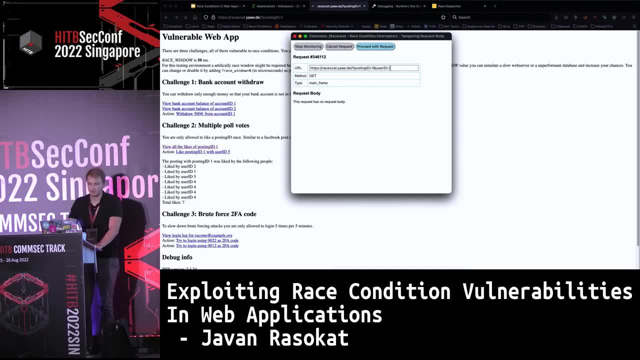 which is the proof of conception. I'm now trying to attack the one which is doing the votes. Like I, should be only able to submit one vote for one picture, like one Twitter feed, only once from one user ID. So there's a limitation implemented. 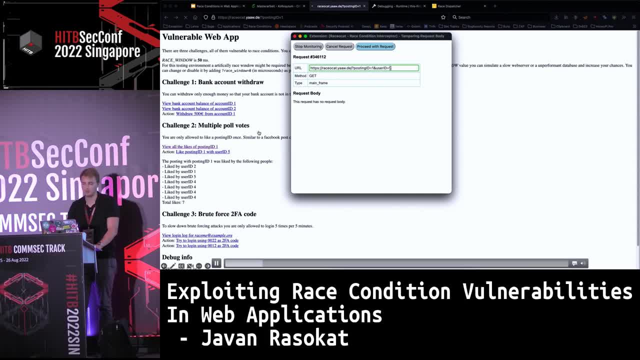 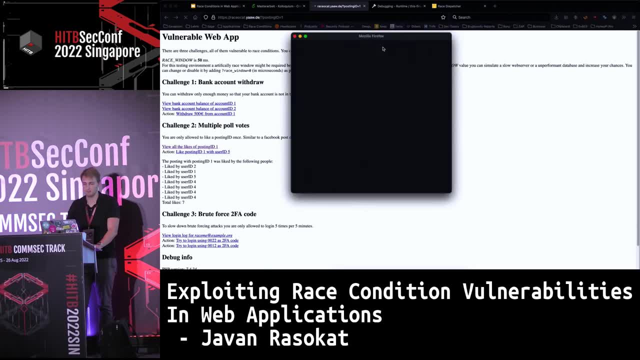 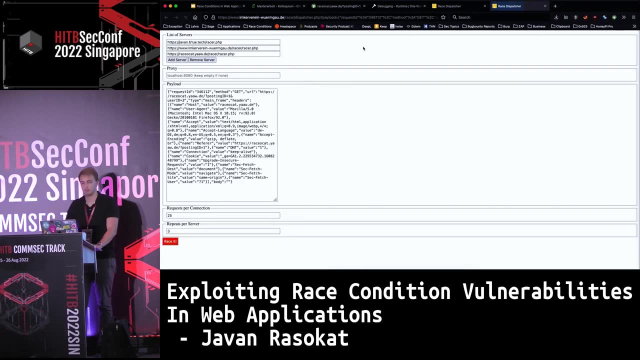 by the business logic of the application And now I am trying to attack that request which is doing this, which is submitting the vote. I'm now forwarding this request to my dispatcher on my race routine infrastructure And you see, there's also a list of servers. 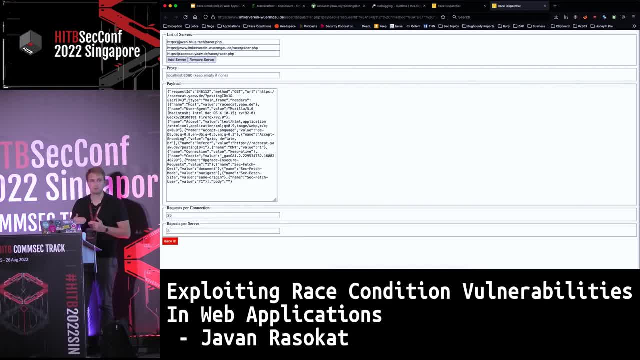 So this is the servers which are going to execute the actual HTTP request to the targets. So now you're on a dispatcher and now we started the racing and here we see it worked. And now I go back to the application And when I refresh the view now I see I was able. 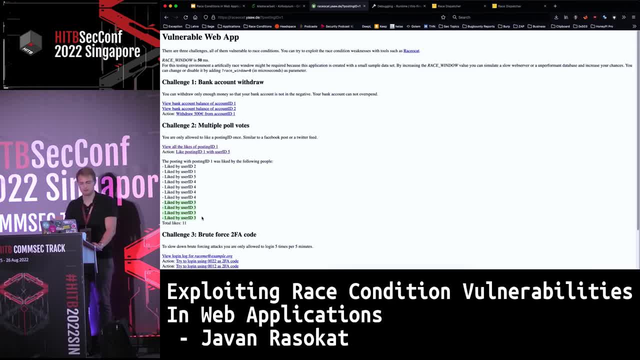 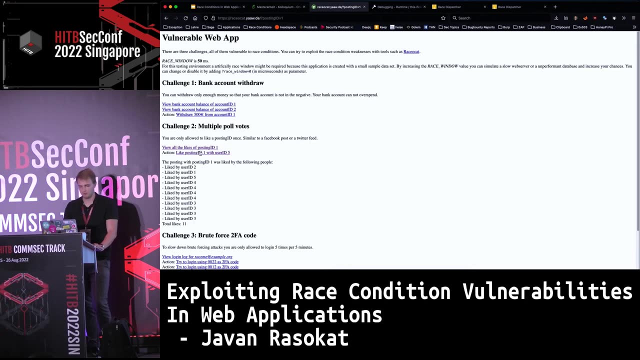 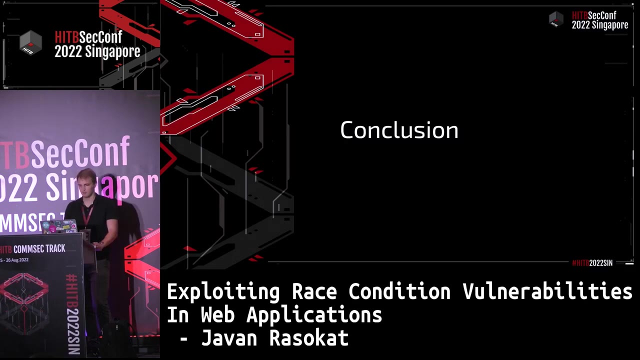 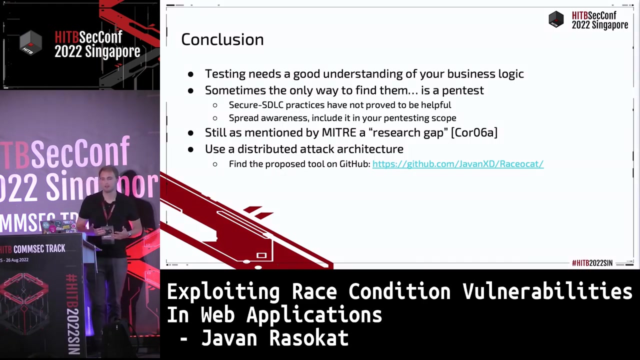 to submit multiple likes from the same user ID. So I was able to bypass this limitation: submit multiple likes by one user ID. So this demo that worked. Let's come to the conclusion. Testing of race condition needs a very good understanding of your business logic. 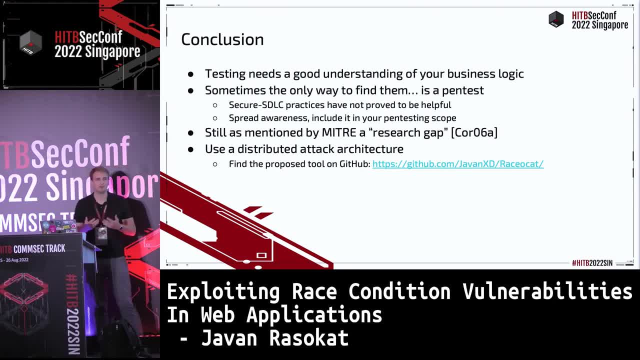 You need to know which places did make sense to exploit it, to get some benefit from it, And we saw that the only way to find them really can sometimes be only a penetration test or by using a manual attack tool with proof-of-confidence. 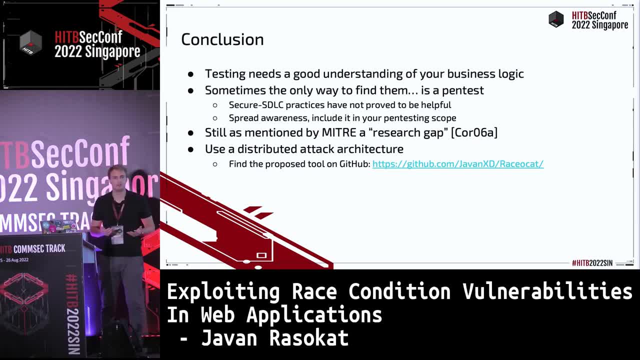 With proof-of-concept, proven that secure SDLC practice do not always help. We still need a human to do this job And I want to spread awareness about this type of vulnerability. That's why we are having this talk, also Because I think race condition. 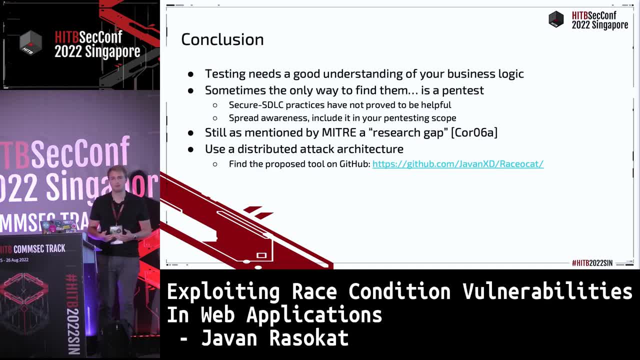 is a very underestimated topic. It can do harm And I think there are still a lot of applications out there vulnerable to this. It's just so little known about this. Like Maito mentioned, it's a research gap And everyone is talking about OWASP top 10. 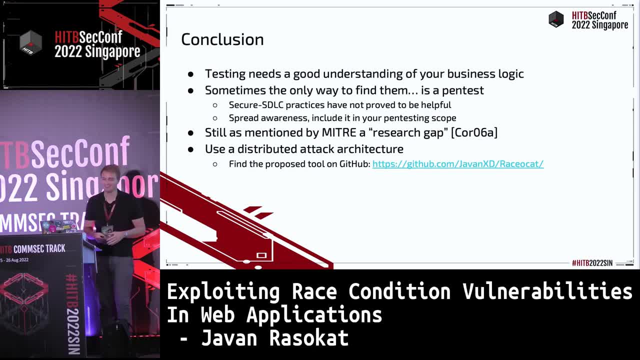 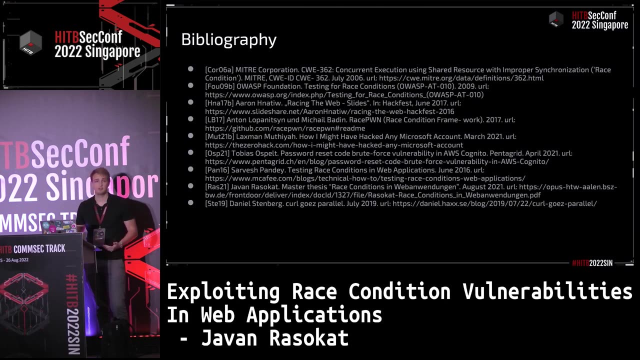 and testing for them, But not exactly the same with race conditions. And also there's- yeah, use the proposed ATT&CK tool with a distributed architecture. You can find this on GitHub. So thank you very much. If you have any questions, I am happy to take them. 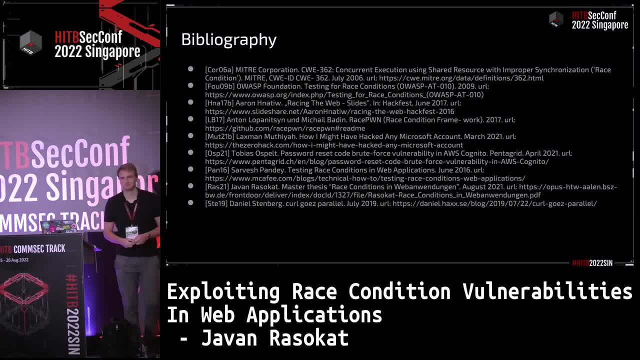 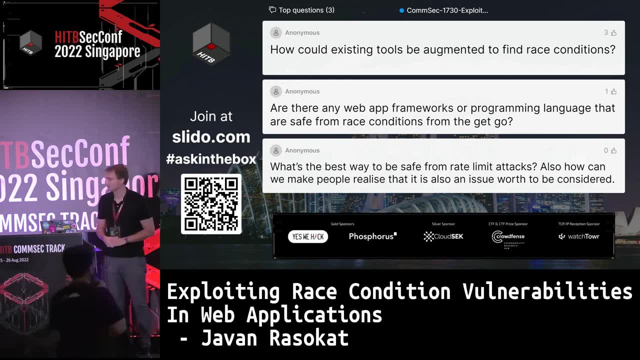 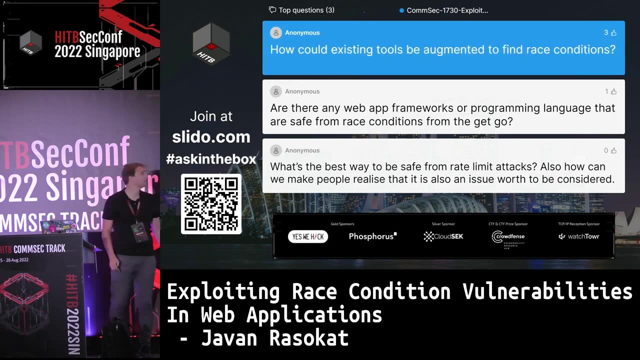 Thank you, All right, so first question. May I know who asked the first question? Raise your hand, please. All right, please proceed to the back to receive your prize First. how could existing tools be augmented to find race conditions? 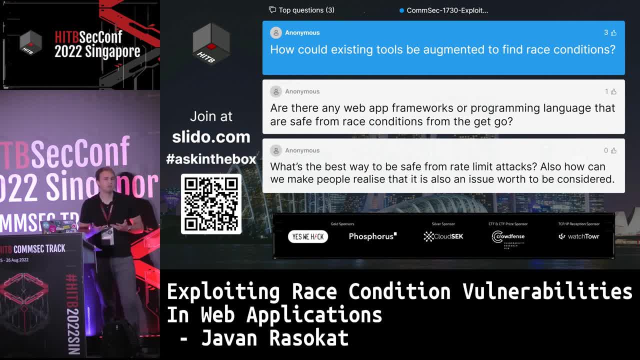 Yeah, my tool is based on the existing tools of their knowledge. I just improved what they did by using more server and they do. But they do their job and you can use them to find race conditions If the target service maybe has bigger time delay. 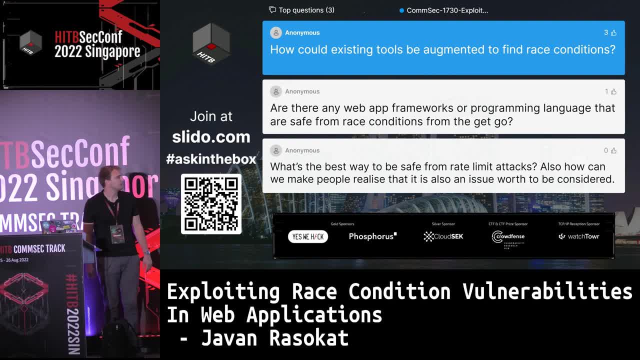 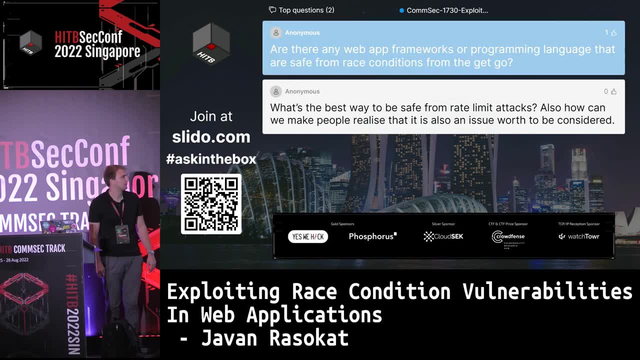 So yeah, Okay. Next, are there any web app frameworks or programming languages that are safe from race conditions from the get go? I don't think I don't know Any, because you work with threads or multi processed language nearly everywhere. 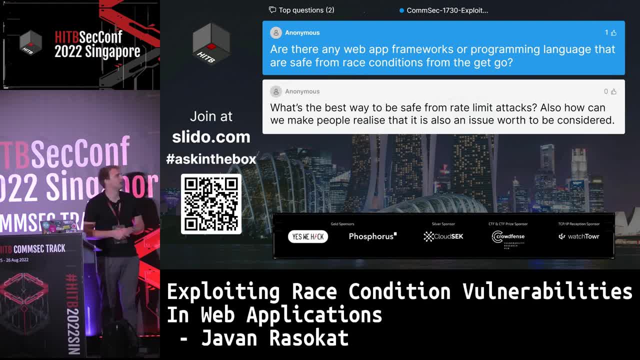 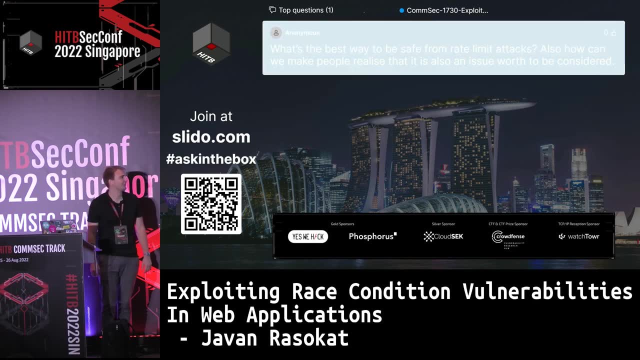 everywhere. and yeah, there are prevention techniques for every programming language. yeah, so I don't know. All different, right, so, Yeah, all different. yeah, Alright. next, what's the best way to be safe from rate limit attacks? 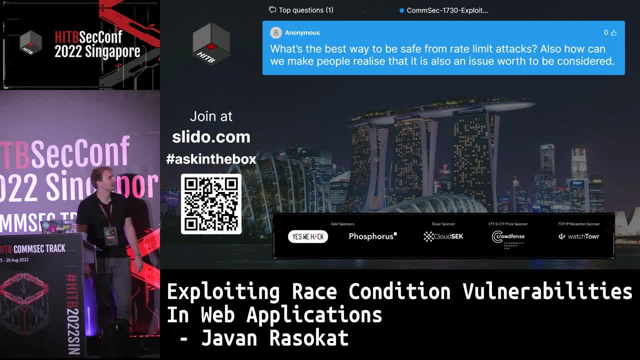 Also, how can we make people realize that it is also an issue worth to be considered? Yeah, it depends how safe your rate limiting is, because we saw some examples that a rate limit was able to be bypassed. so, yeah, maybe. 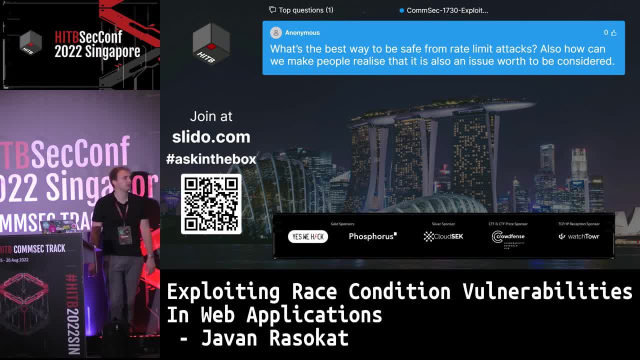 depends on the type of rate limit that this is safe from. the rate limit must be safe from race conditions first and, yeah, I try to share awareness about this vulnerability by having this talk, so that's, I hope that we can make people aware. yeah. 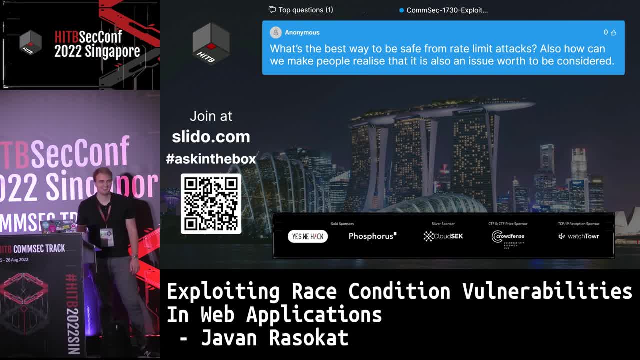 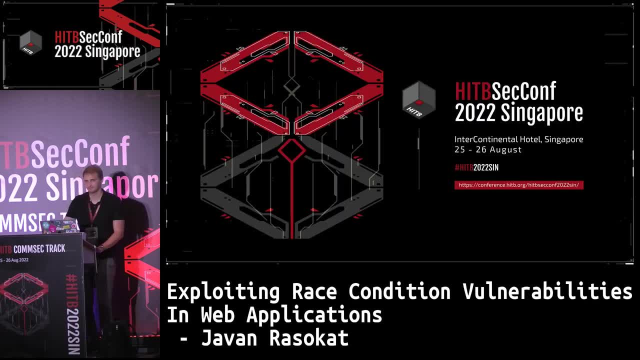 Alright, if there are no further questions, could we give a hand for our last presenter? Yeah, thank you. Thank you very much, so we have actually come to the end. oh sorry, one more question. Yeah, we have one more question. 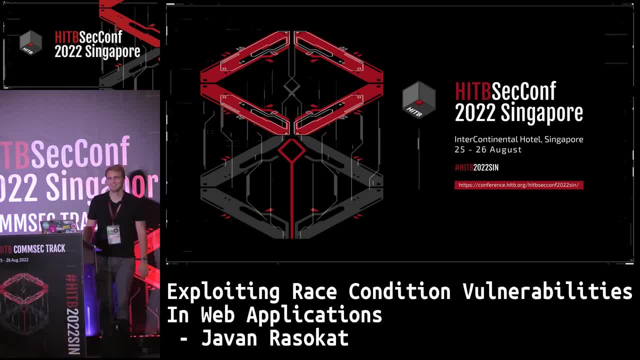 Alright, sure, let me hand you the mic. Now it's live, so let's try to be back in the previous conference where we have live questions. Yeah, So thanks to you. thanks so much for the presentation, and I just would like to know if you try to make. 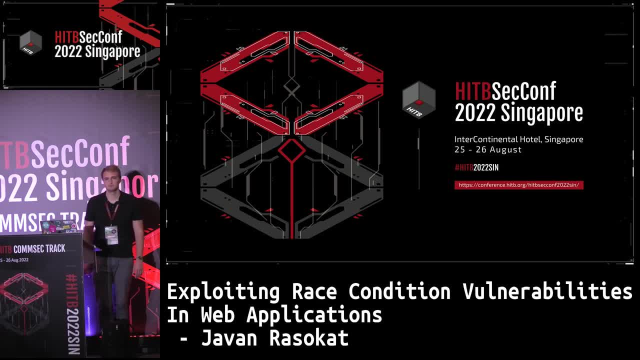 race conditions to different backends. so usually it's happening with a statement and update in some DB. so we have several technology with databases and no SQL, not whatever. so did you try to see if there is some of them that more robust against race condition?